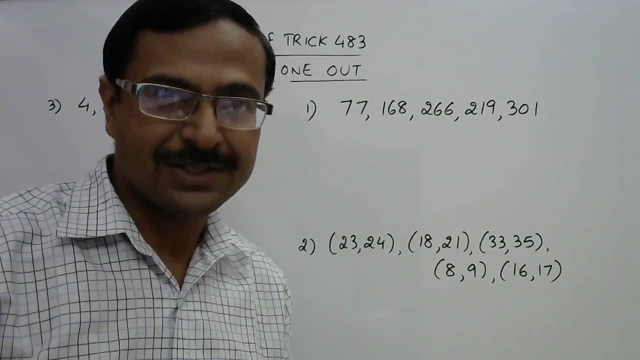 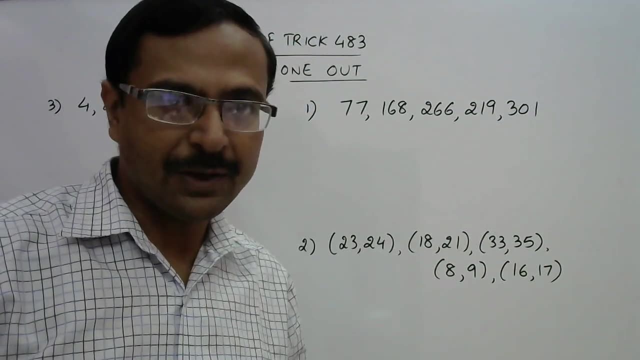 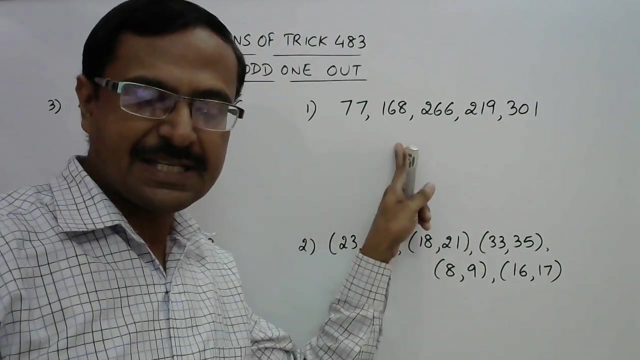 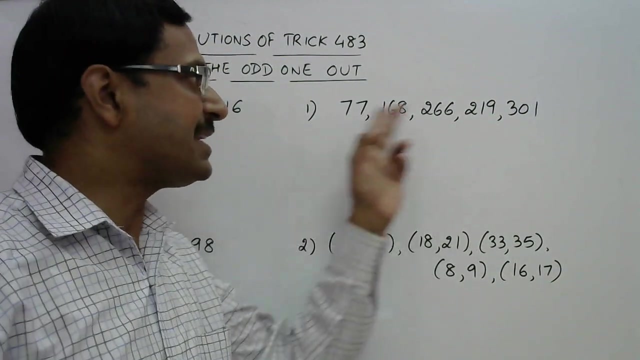 and many of you got all four correct, So that was very heartening to see. but just for the convenience of others who could not solve it here I go with all the four solutions Now. the first question was 77, 168, 266, 219 and 301.. Now, since the numbers vary from 77 to 301, you need to check. 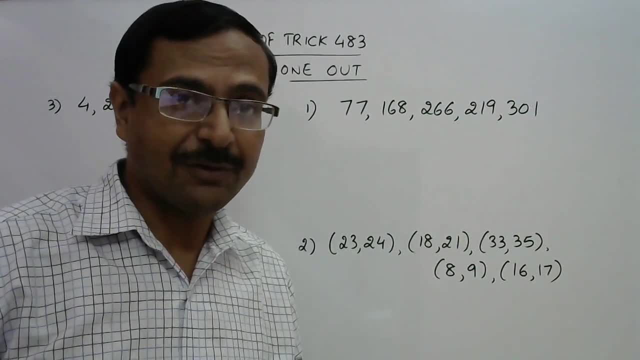 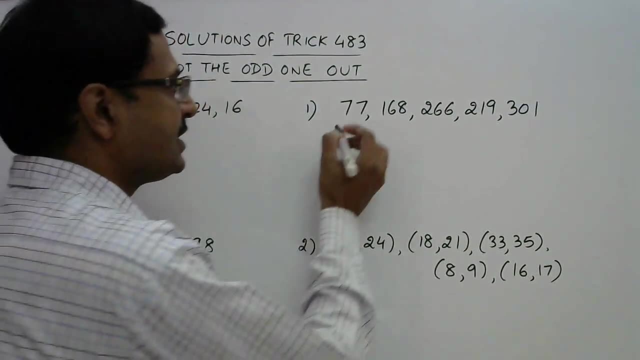 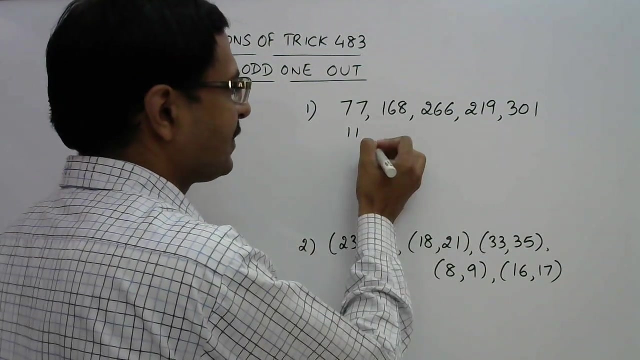 the divisibility, and divisibility by 7 is one of the most important things. So I am going to talk about the toughest thing. So you need to check all the numbers whether they are divisible by 7 or not. See, 77 obviously is divisible by 7.. 7 into 11 is 77. If you check this, 7, 2s are 14. 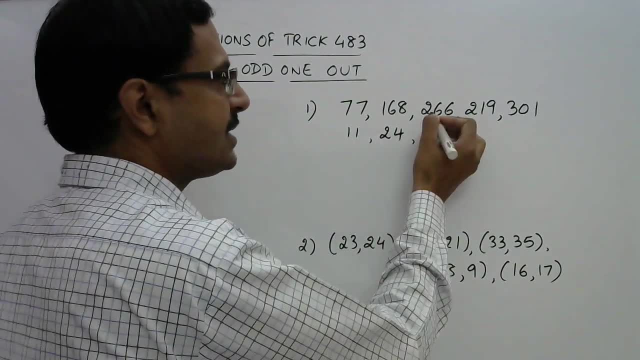 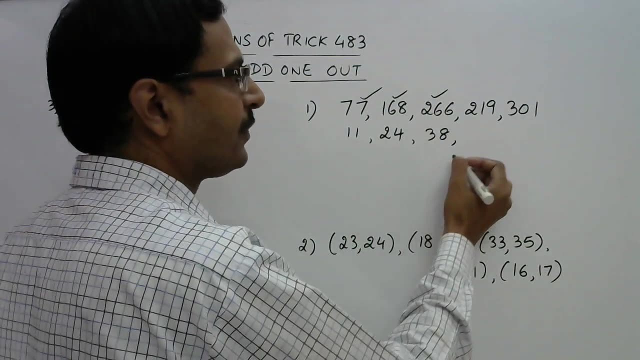 and 28. So 7, 4s are 28.. 7, 3s are 21. So 56, 7, 8s are 56. So all three are divisible. But in this case this is not divisible. 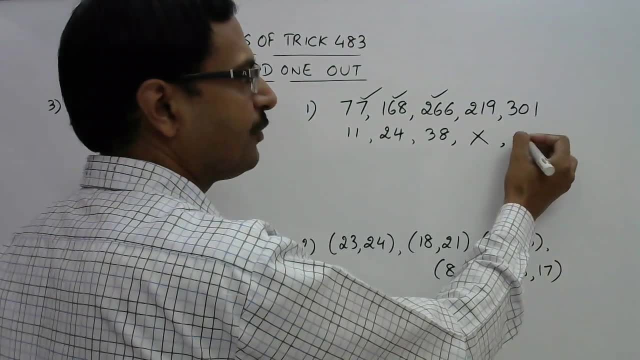 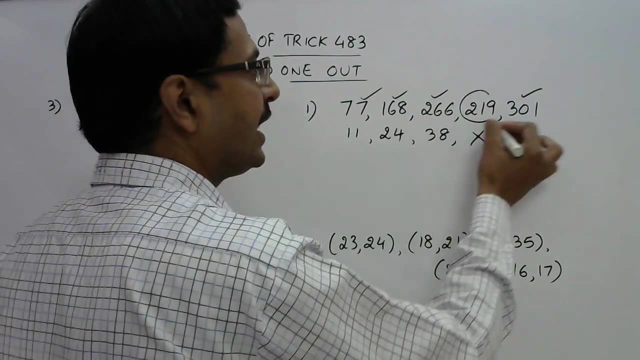 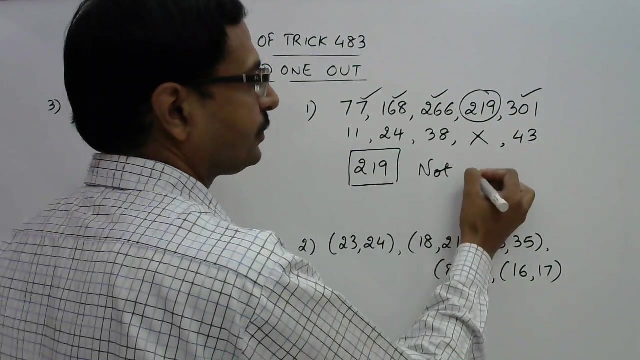 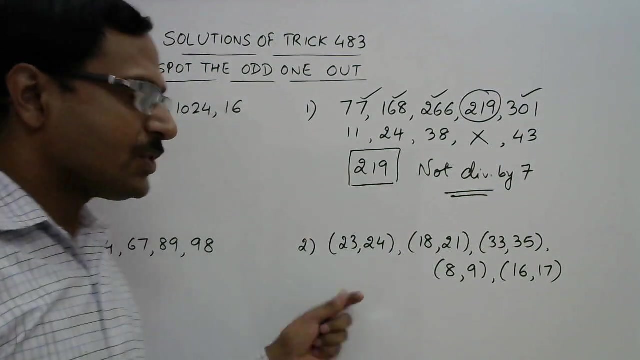 And finally, 7, 4s are 28,, 21,, 7, 3s are 21.. So four numbers are divisible by 7, but 219 is not divisible by 7.. So 219 is the answer. This is the reason for this answer In the second question I gave you. 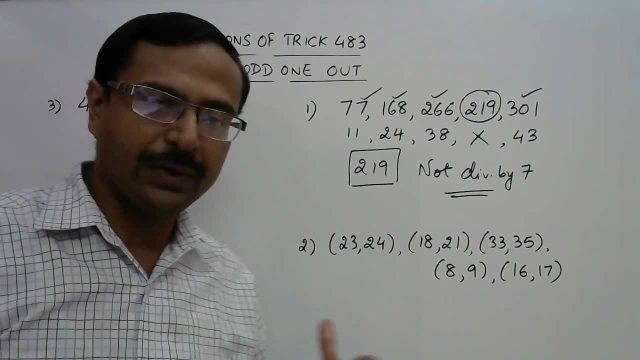 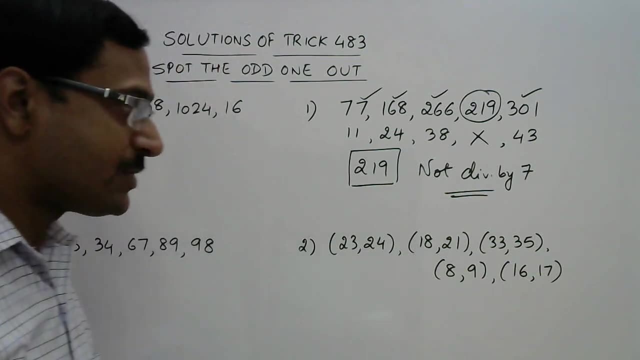 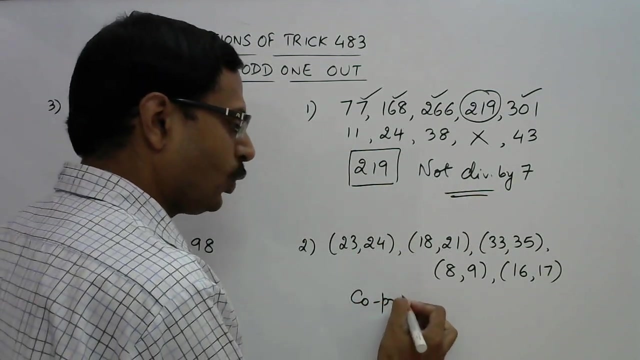 five pairs of numbers and you needed to find the odd one out. Whenever you have pairs of numbers, then you have to link the two numbers in the bracket. Now see, observe carefully that 23 and 24 are co-prime. Co-prime numbers are those numbers. 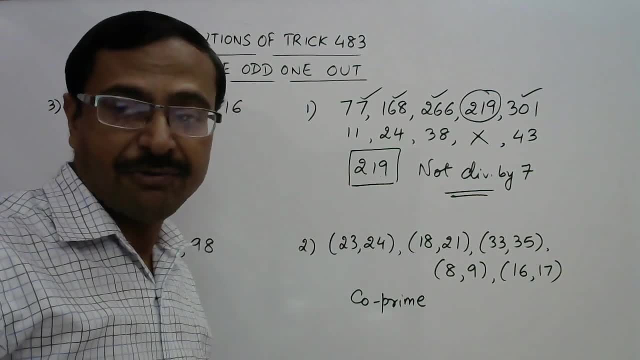 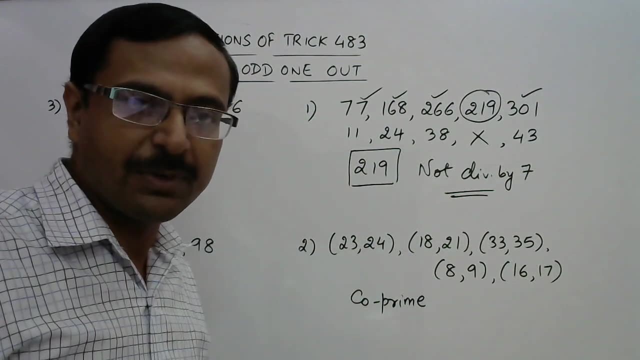 which have hcf1. That is, they do not have any other common factor except 1.. Obviously, 1 is a factor of every number, So 23 and 24,. 23 is a prime number, So it cannot have. 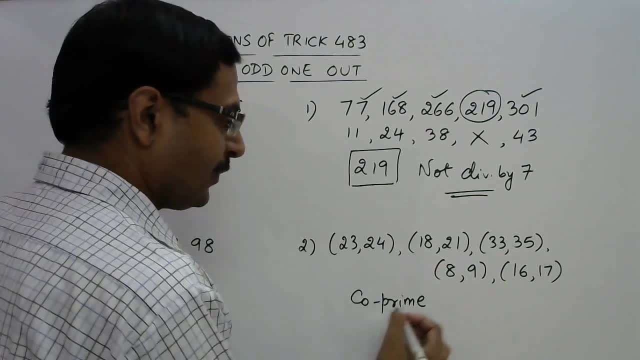 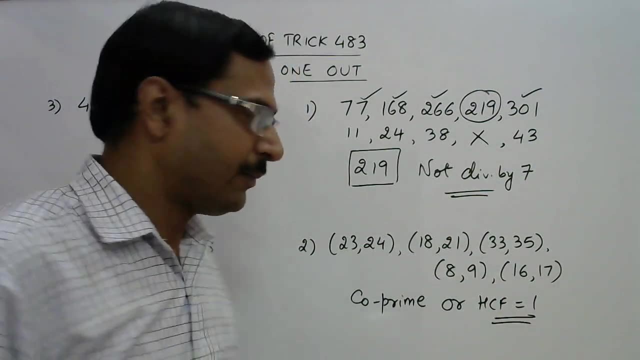 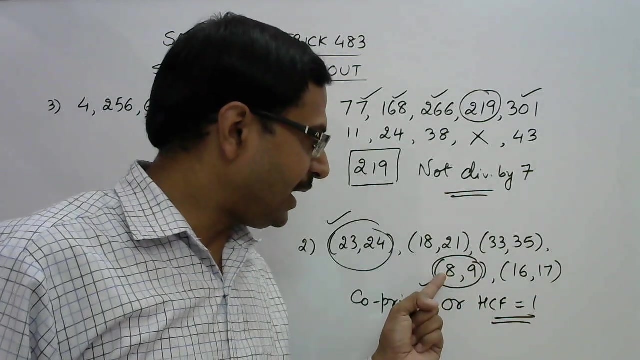 which is common to 24.. So they are co-prime, Or hcf is 1.. So no common factor other than 1.. So these are co-prime, Correct. 8 and 9 obviously are co-prime because 8 is having. 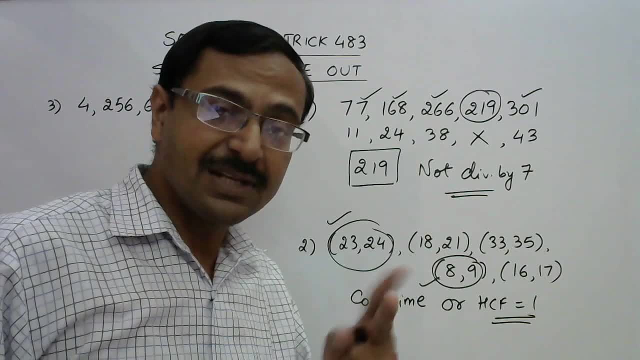 all factors 2 into 2 into 2, and 9 is having factors 3 into 3.. So no common factors. 16 and 17,. obviously they are co-prime because 17 is prime, So one of the numbers is prime. 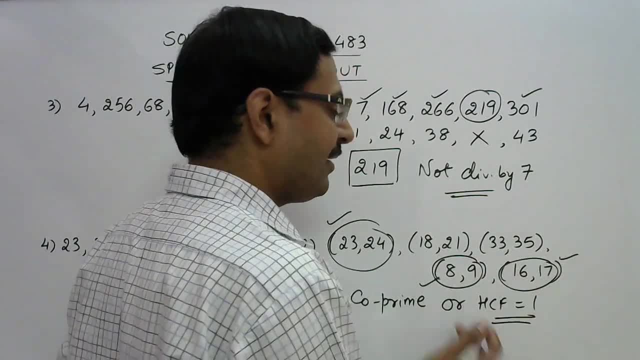 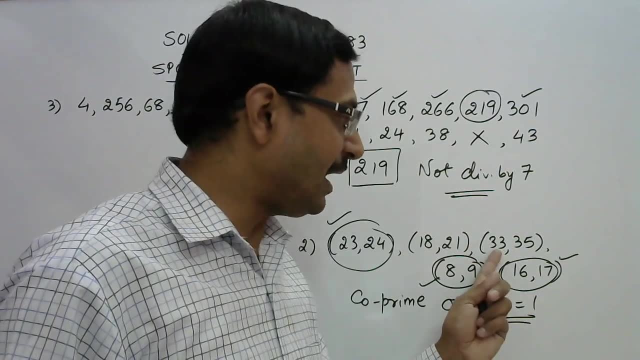 means 33 and 35,. 33 is 3 into 11.. So factors are 3 and 11.. But in case of 35, we have 5 and 7.. So 3,, 11,, 5, 7, all factors are different, So these two numbers are also co-prime. But. 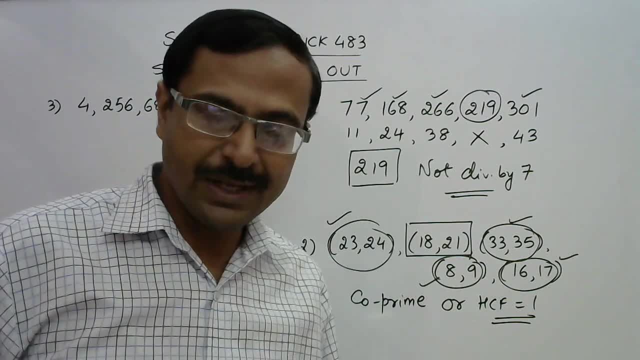 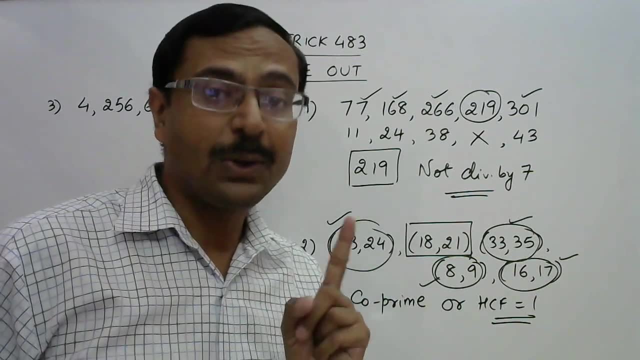 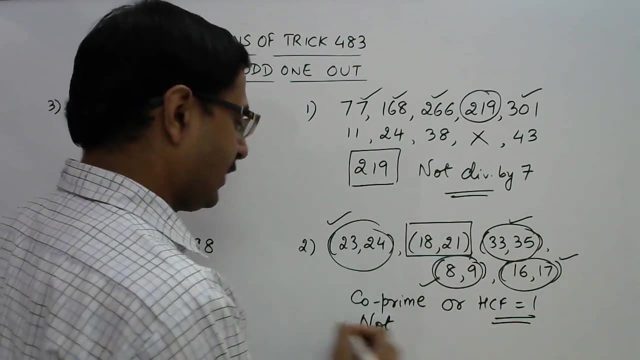 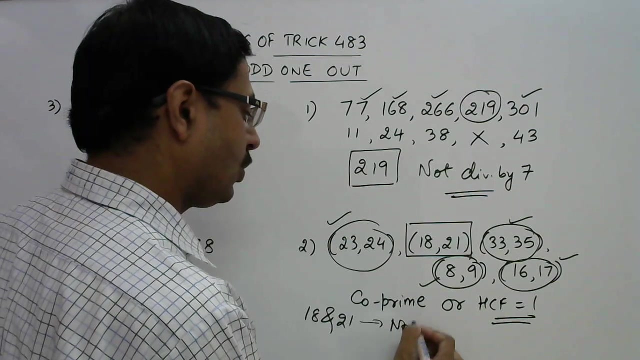 in case of 18 and 21,. they are divisible by a common number, 3.. So 3618, 37021.. So they are not co-prime. So this is the odd one out 18.. 21, just because they are not co-prime. So 18 and 21 not co-prime, Or they have a common. 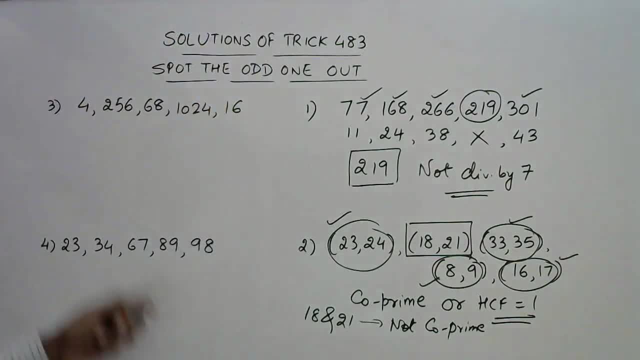 factor other than 1.. Let us have the third question now. Very simple one: Maximum. people got this one right. See, all are even numbers. But if you observe carefully, 4 is 2 raised to the power of 2.. So it can be expressed in the power of 2.. 256, 2 raised to the power. 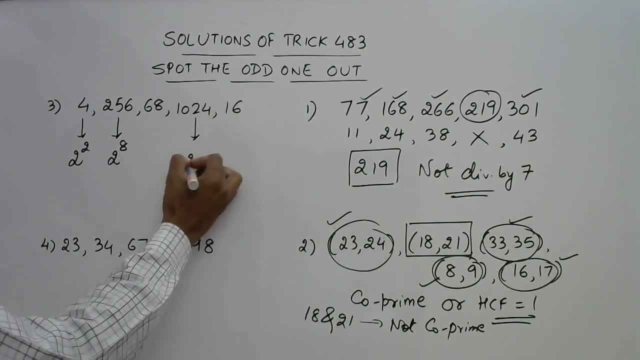 8.. 1024, 2 raised to the power 10.. And 16 is 2 raised to the power 4.. So all numbers can be expressed in the powers of 2. But in case of 68, you cannot express it in the power. 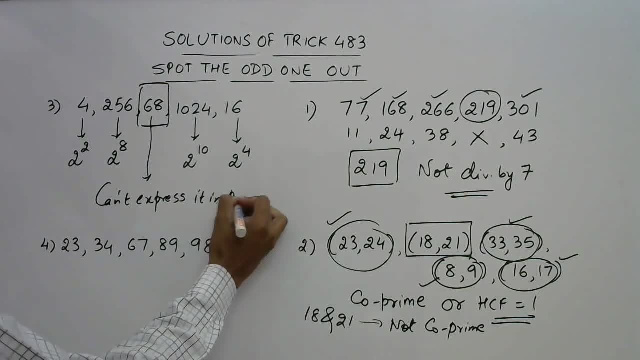 of 2.. So this is the odd one out in this question. 68 is the answer. Let us have the final question: 23,, 34,, 67,, 89 and 98. Now, in this case, all the numbers, just see 23.. It is 22 plus 1.. 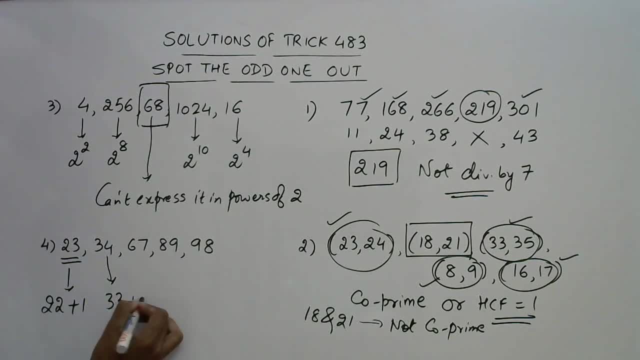 What about 34?? It is 33 plus 1.. What about 67?? It is 66 plus 1.. What about 89?? It is 88 plus 1.. So how we are writing the numbers? These all numbers are doublets, So we are having a doublet plus 1.. This is the rule.